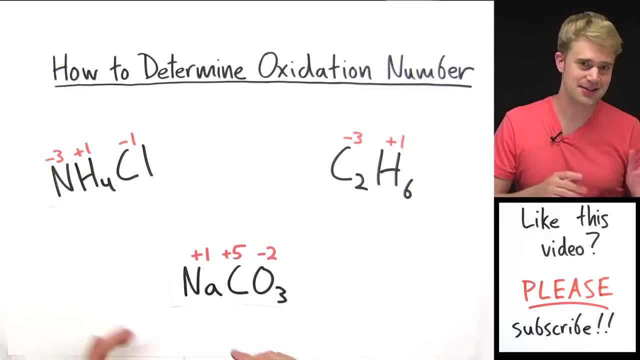 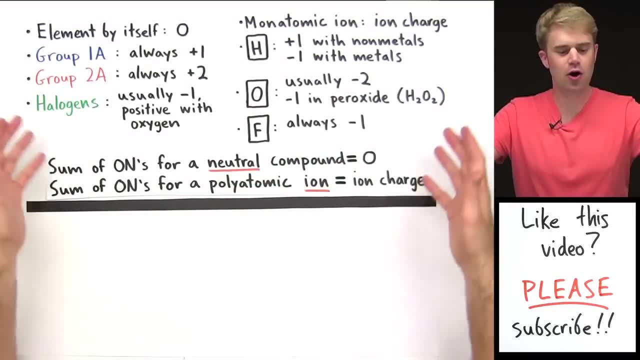 or why they're important. check out my video called what are oxidation numbers. In this video, we're going to work through the process of how you figure out what these numbers are. So here are the rules that we're going to use to figure out oxidation numbers. Now, just so you. 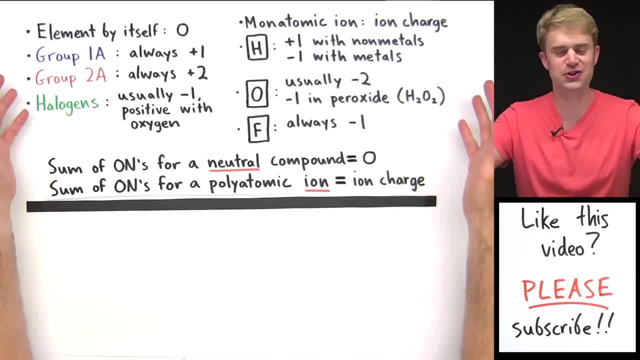 know, every teacher and textbook has their own version of these rules, but they all work in pretty much the same way, So if you learn mine, you'll still get the answer right 100% of the time, even if these are a little bit different from your teachers. I'm going to talk through a few of these. 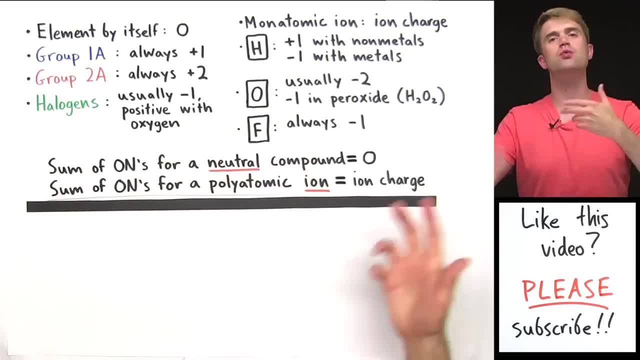 rules right now and then I'll introduce the rest just as we work through practice problems. The first rule is the oxidation numbers. The oxidation numbers are the numbers that we're going to use to figure out the oxidation numbers. The oxidation numbers are the numbers that we're going to use to figure out the oxidation numbers. 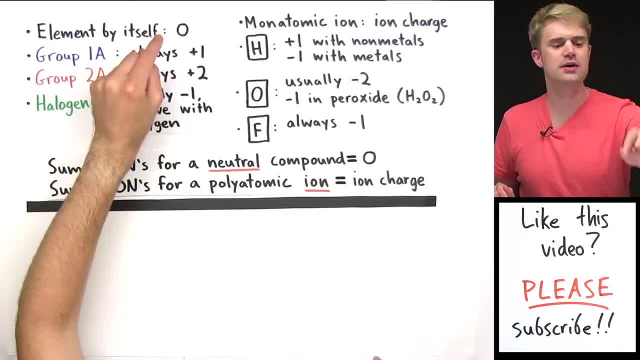 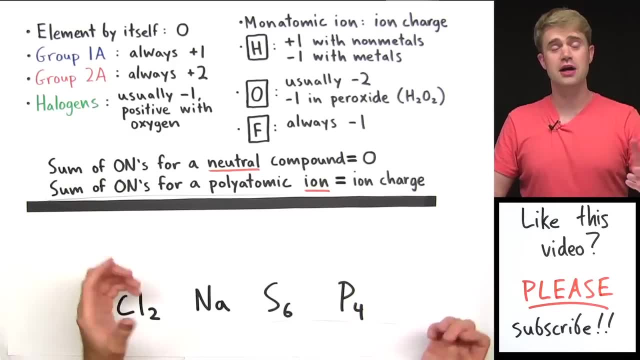 The first is this: An element by itself always has an oxidation number of zero. Here's what I mean by that. There are a lot of chemical compounds that have just one element. That element is not combined with any other elements. That's what I'm calling an element. 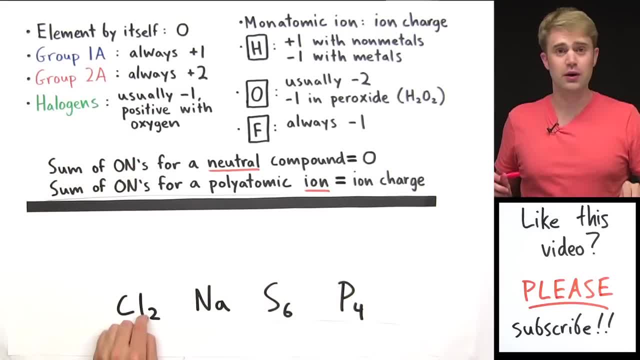 by itself. So that's something like Cl2.. It doesn't matter how many atoms of that element you have, just as long as it's only that element and none others. So Cl2: an element by itself, oxidation. number of zero. Sodium, Na by itself zero, S6, just sulfur, nothing else. 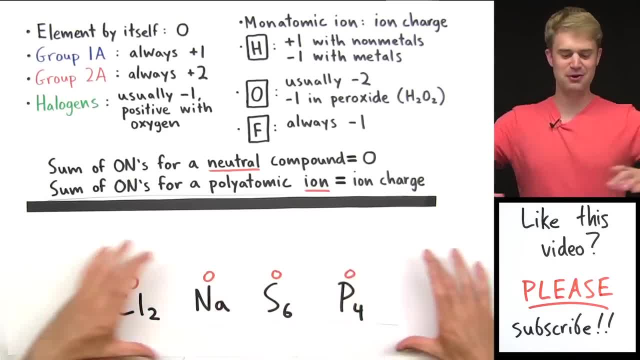 P4, phosphorus and nothing else- zero. So that's probably the easiest rule here. It's always zero for the oxidation state if you have an element by itself, with nothing else. The other rule here is about monatomic ions. These are ions that are made of only one atom, So like this: 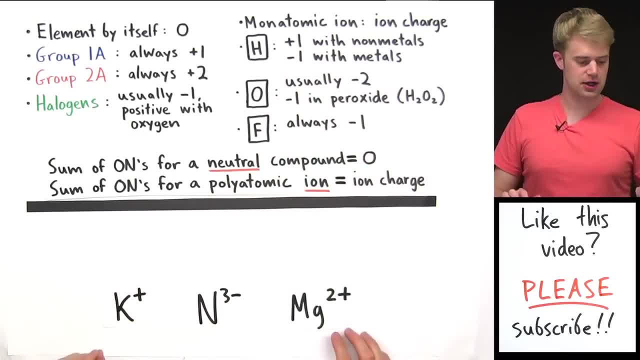 For monatomic ions, their oxidation number is the same as their ion charge. So for K plus here its oxidation number is going to be plus one. For N3 minus, it'll have an oxidation number of minus three, And Mg2 plus here is going to have an oxidation number. 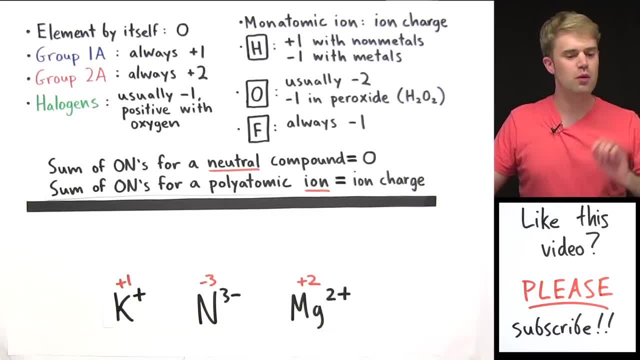 of plus two. Now keep this in mind: When we write oxidation numbers, we write the sign first, So plus, minus, and then the number after. This is the opposite of how we write ionic charges. So just keep that in mind. The charge might be two plus on magnesium, but the oxidation number is plus two. 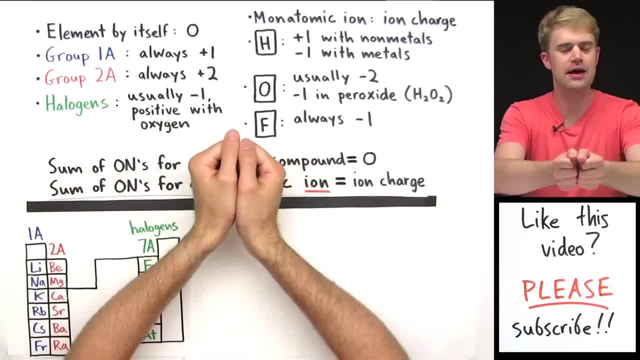 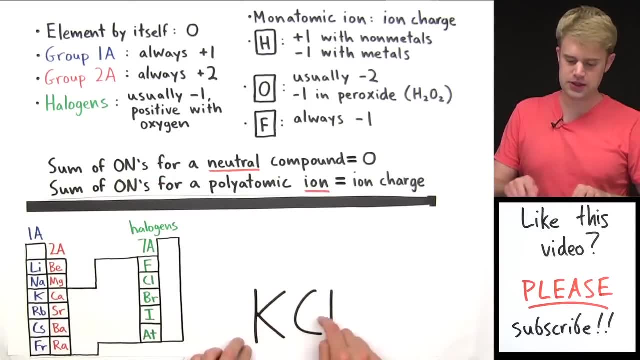 Now for the rest of these rules. we usually use more than one together, So I'll just talk about these as we use them in example problems. Here is our first example: KCl. we want to figure out the oxidation numbers of the elements in this. 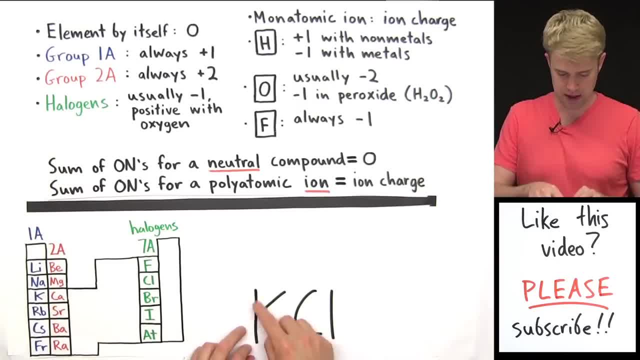 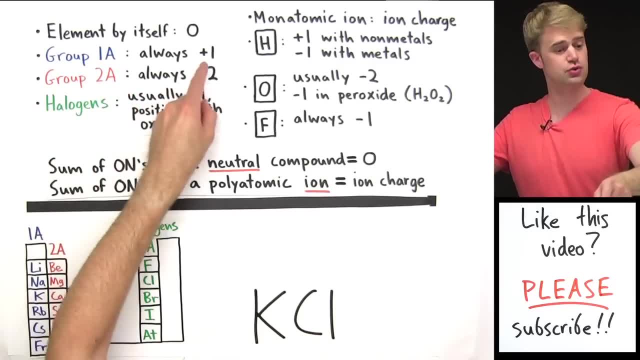 compound. So for KCl, we want to figure out the oxidation numbers of the elements in this compound. OK, so let's take a look at our rules here. K potassium is in this column in the periodic table. It's in group 1A, So there's this rule that elements in group 1A are always plus one. 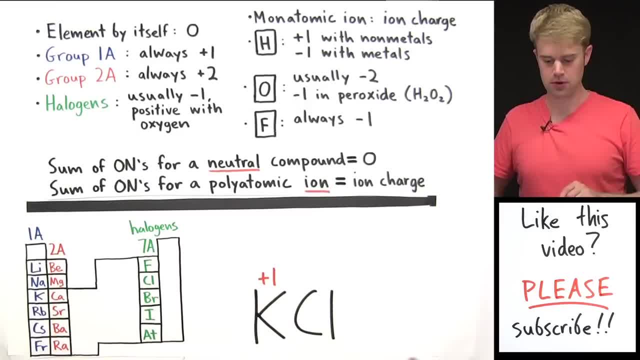 So that is potassium's oxidation number. Then we have Cl over here. That is one of the halogens. Halogens usually minus one positive with oxygen. Well, Cl certainly isn't with oxygen here, So we'll give it a minus one oxidation number. Now I want to use this to show you a third rule. 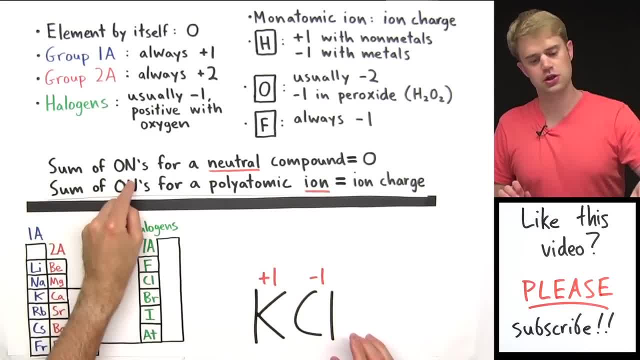 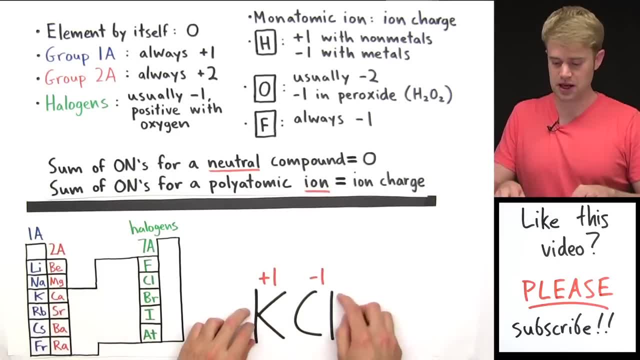 That's this rule. right here, The sum of oxidation numbers for a neutral compound equals zero. KCl is a neutral compound here. It doesn't have a charge after it. So that means that the sum of these oxidation numbers is going to equal zero, And that's definitely true here. 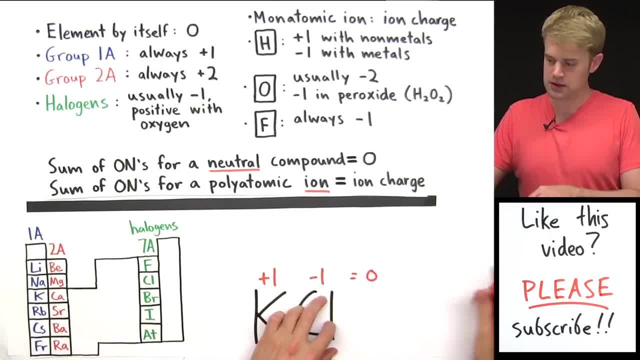 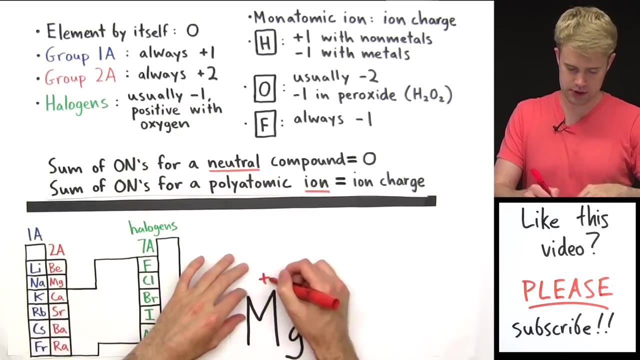 Plus one minus one equals zero. We'll use this later on when we do other examples, But just keep that in mind. The sum of oxidation numbers for a neutral compound should always equal zero. MgO- Mg is in this column in the periodic table. group 2A And group 2A elements are always plus. 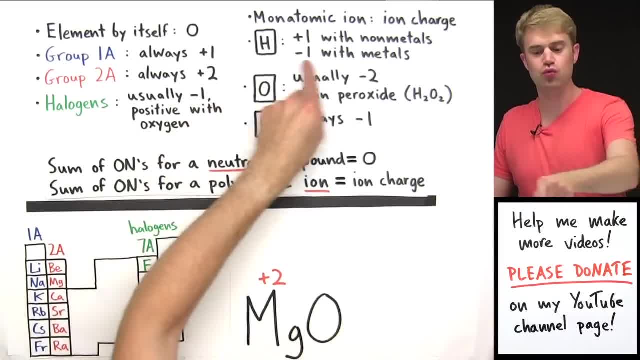 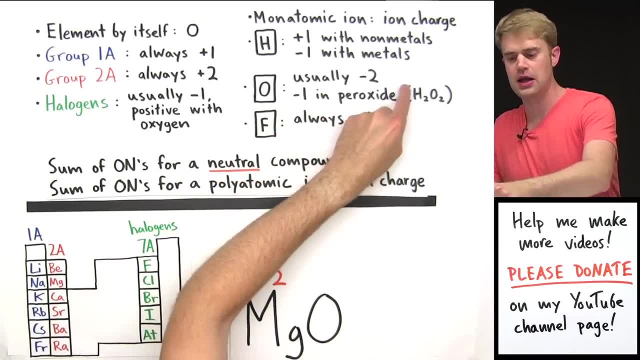 two. So there's that Oxygen here. we have a rule for oxygen: It is usually minus two. It is minus one In peroxide, H2O2, hydrogen peroxide is the most common peroxide. It's probably the only one you'll. 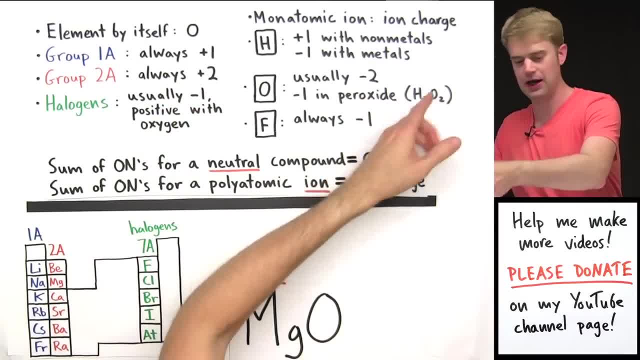 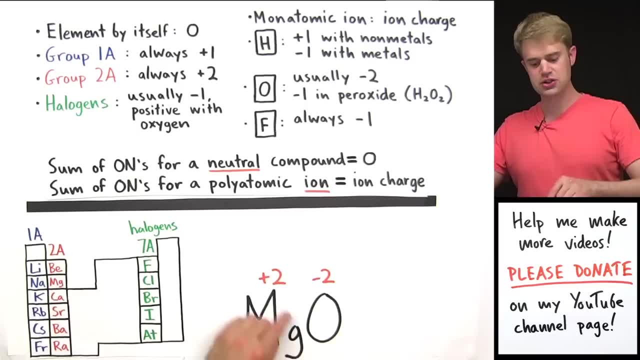 ever see. But anyway, this oxygen is definitely not in hydrogen peroxide, So it's fair to say that its oxidation number will be minus two, Plus two for Mg, Minus two for O, And they add together to make zero, because this is a neutral compound: CO, carbon monoxide. Let's figure this one out. 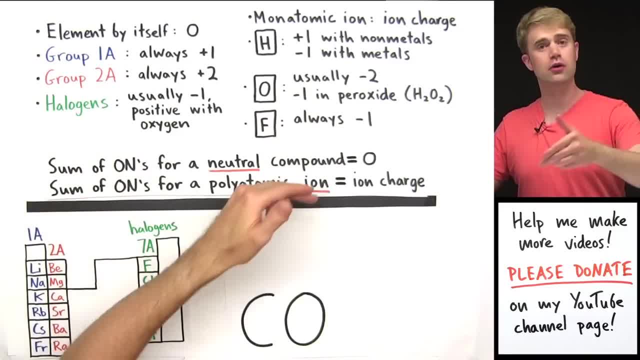 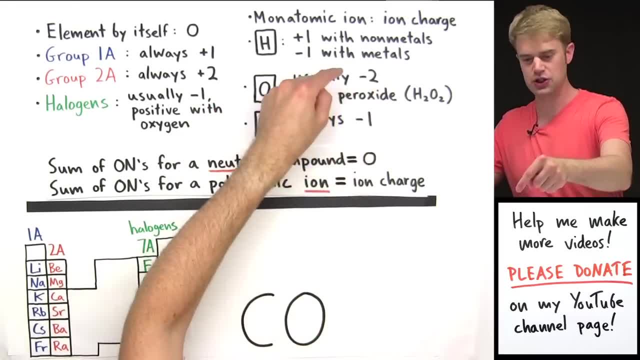 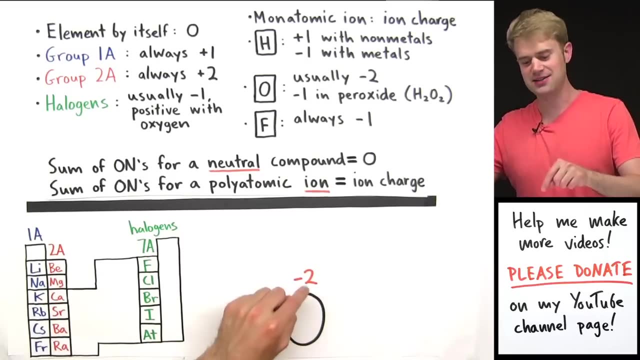 So see, here there isn't any rule for carbon, So we'll have to figure it out based on what we do know. So we do know oxygen. Oxygen is usually minus two, unless we're in a peroxide- Definitely not a peroxide- So we can safely say that oxygen's oxidation number is minus two. Now let's use this. 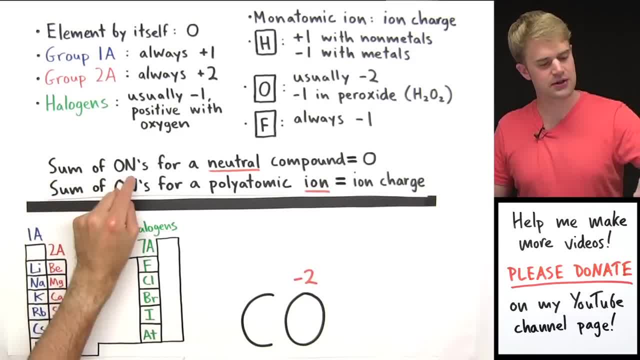 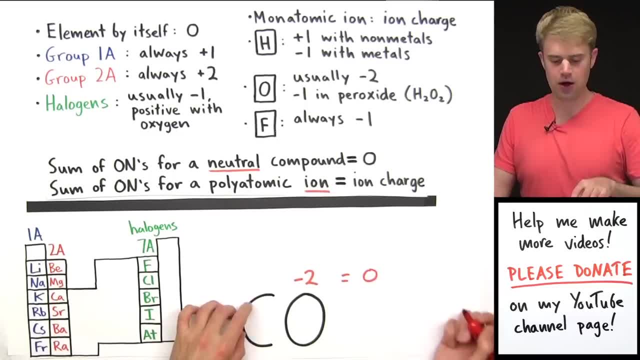 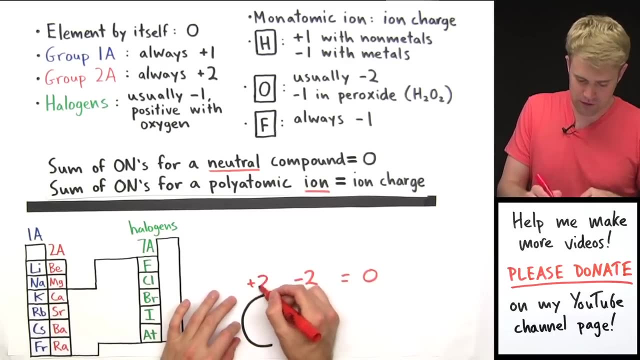 other piece of information that we know And that's the sum of oxidation numbers for a neutral compound should equal zero. So whatever carbon's oxidation number is should add together with oxygens to make zero. So we can figure out that carbon's oxidation number should be plus two. 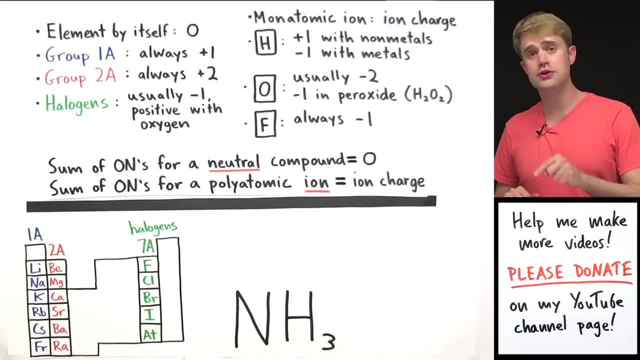 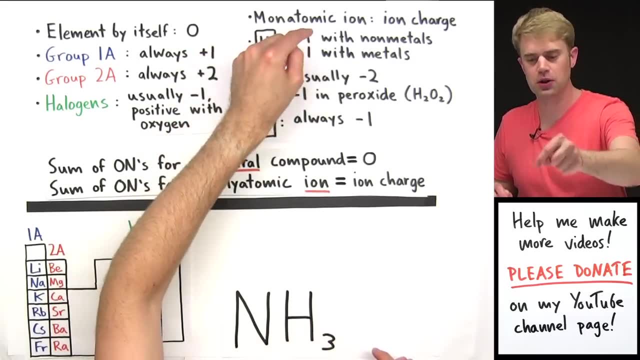 Minus two from oxygen gives us zero NH3.. Okay N? there isn't any information about that. So, just like in the last example, we'll have to figure out its oxidation number using what we do know. Here we've got hydrogen. There's a rule for hydrogen: Hydrogen is plus one with nonmetals. 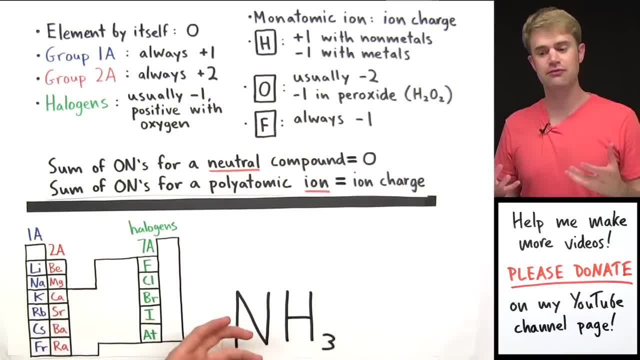 and minus one with metals. So nitrogen is definitely a nonmetal, which means that in this case, hydrogen is going to have a plus one oxidation number. Okay, But there are three hydrogens. Each one of them has a plus one. So what we have to do is we have to multiply this plus one times. 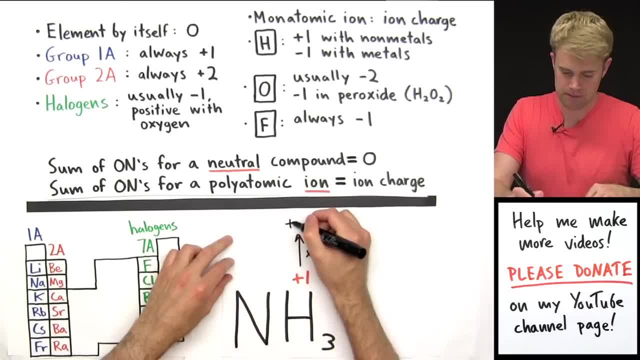 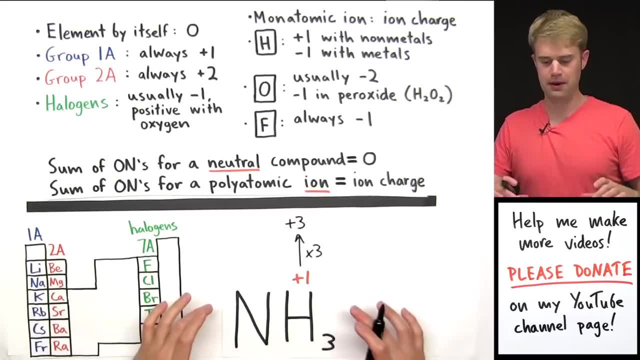 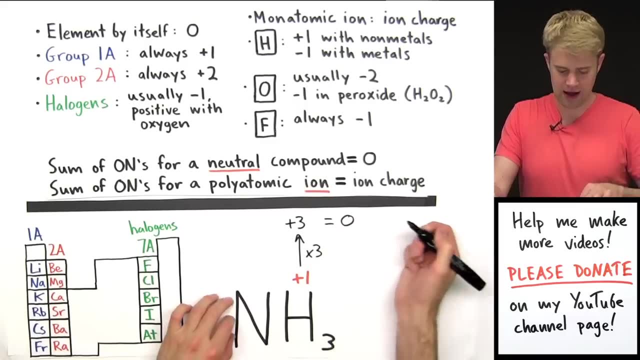 for the three hydrogens, and that's going to give us plus three. Now let's keep this rule in mind: that the sum of oxidation numbers for a neutral compound should equal zero. NH3 is definitely a neutral compound. We don't see any charge here. So whatever nitrogen's number here is needs to. 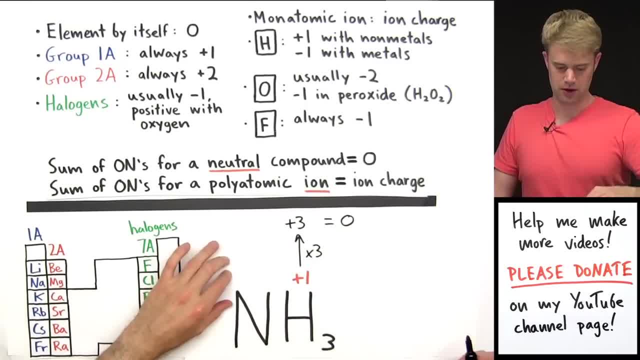 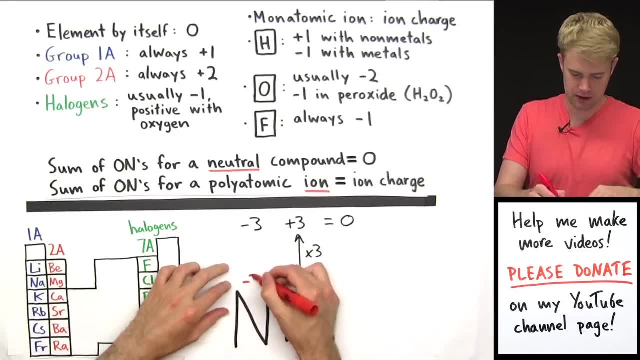 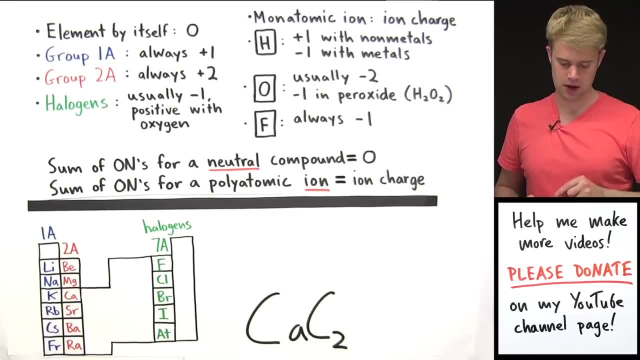 add together with plus three to make zero. So that means that nitrogen here has to be minus three. That adds there to get zero. So its oxidation number is minus three. Hydrogen's is plus one, CaC2.. So calcium here is in this. 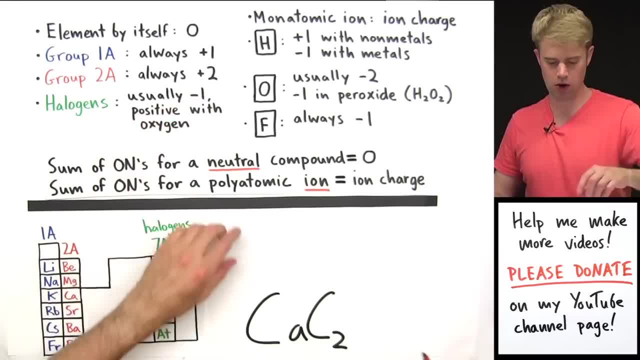 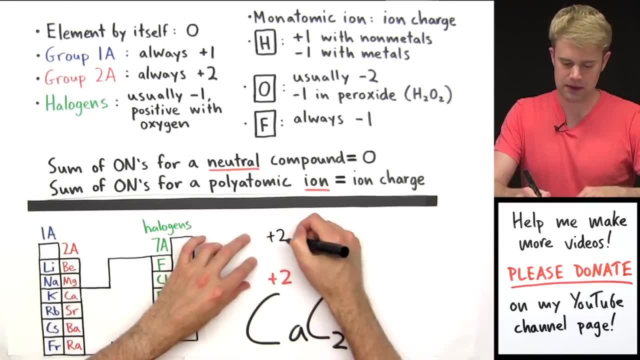 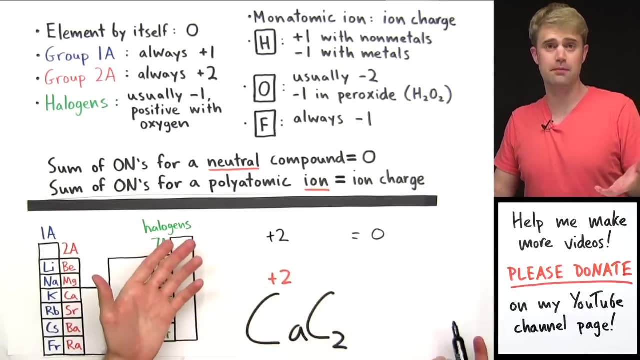 column group 2A. So we know that its number is always plus two. We don't know what carbon's number is, but we can figure it out. What we do know is that calcium's number plus whatever carbon's number is needs to equal zero, because this is a neutral compound. It doesn't have a charge. 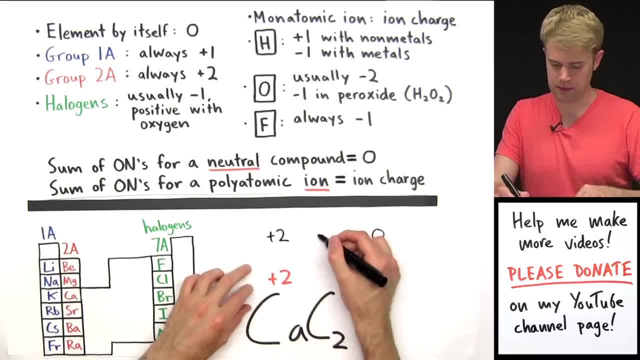 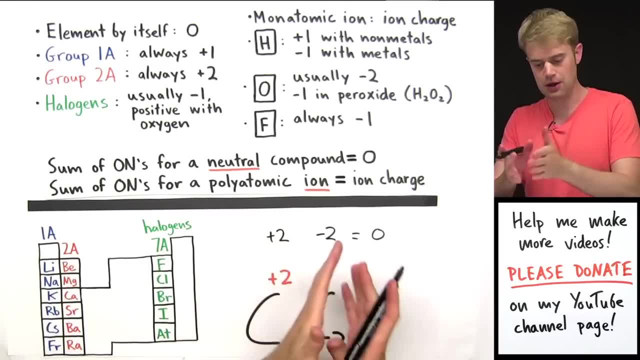 That means that the carbon's number is always plus two. So we don't know what carbon's number is, but we know there's a total number on carbon. Alright, but there are two carbons here, so we have to divide this number between the two of them. So we're going to take this and 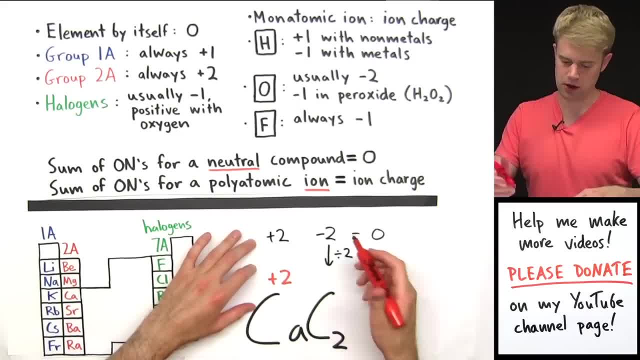 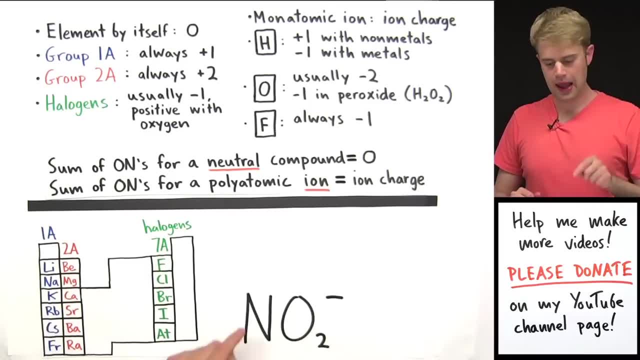 divide it by two to get an oxidation number of minus one for each one, plus two for calcium, minus one for carbon. NO2 1- is an ion. So this is going to be a little bit different. In this case I will be taking something that's less than the number of ions, so N2 is less than 1.. We will be. dividing this number into the number of cultural items and that gets squared. And now if I put this number over here, over here, it would be 3.. And if I begin here, it would be minus 1.. I'm not going to get. 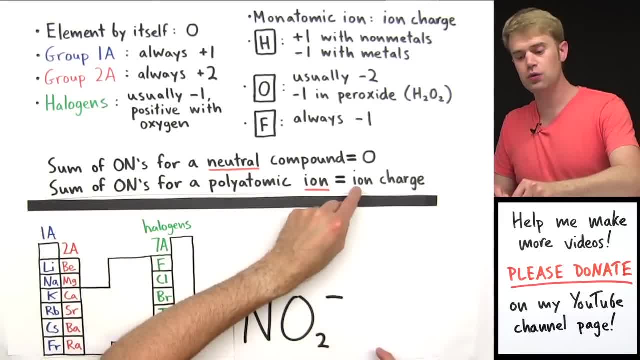 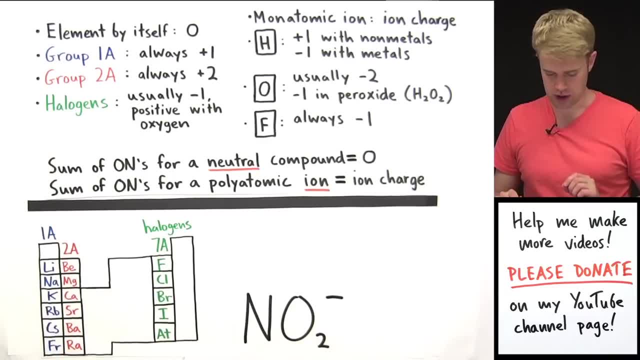 Oxidation numbers for a polyatomic ion equals the ion charge, So let's see how we'll use that here. nitrogen: we don't know what its oxidation number is going to be, but oxygen here is Usually minus 2, so we have minus 2 here, but we have 2 oxygens, So we're gonna do minus 2. 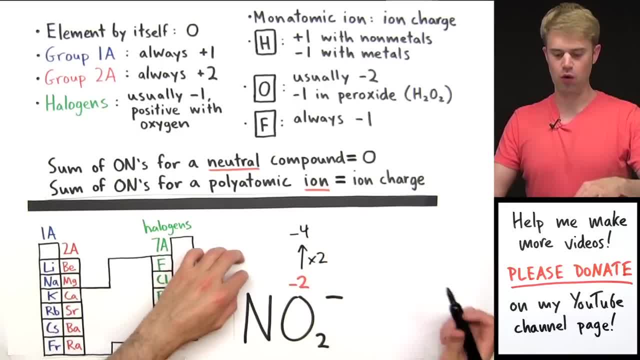 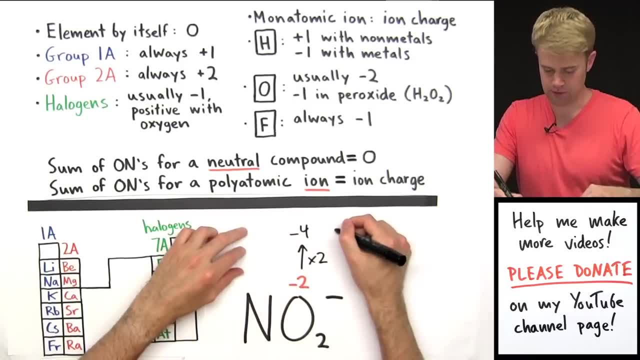 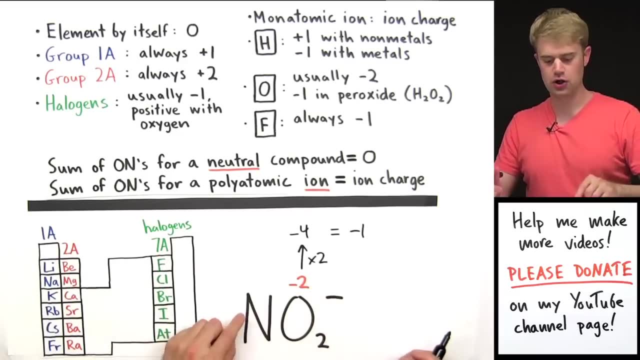 Times 2 is going to give us minus 4 altogether. Now, whatever nitrogens is, when we combine it with minus 4, We need to get not 0, but we need to get minus 1, because that's what the ion charge of NO 2- 1 minuses. 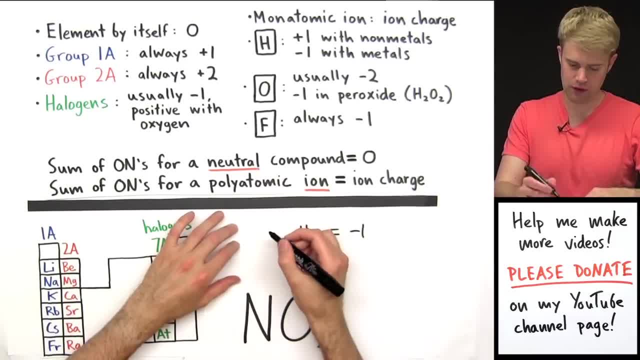 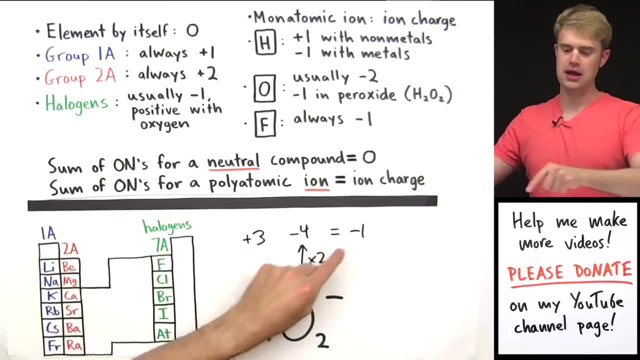 So this means that we will have 3 plus 3 plus 3 minus 4 gives us minus 1, which means that oxidation number here on Nitrogen is going to be plus 3 HNO3. Okay, let's take a look at the rules. We got hydrogen. 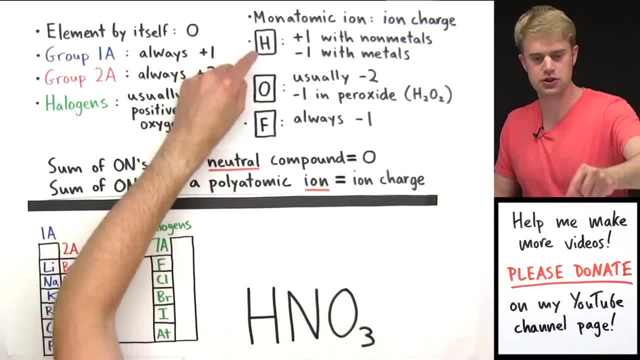 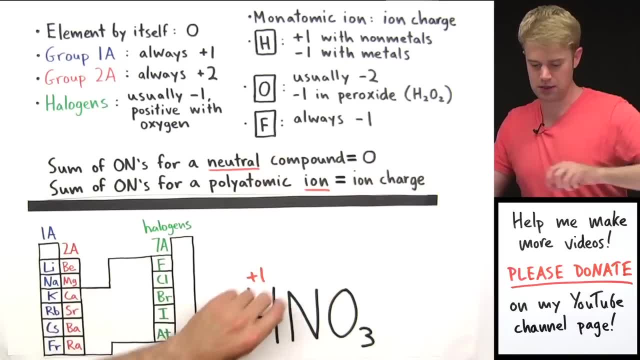 Hydrogen here is combined with nonmetals, nitrogen and oxygen, So that means that its oxidation number is going to be plus 1. Oxygen over here is going to be minus 2, but we have 3 oxygens, So we got to take this minus 2. 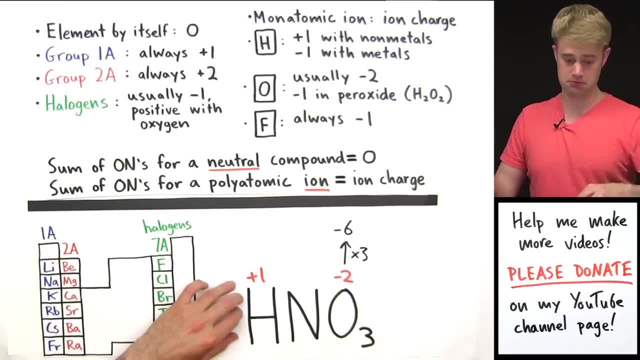 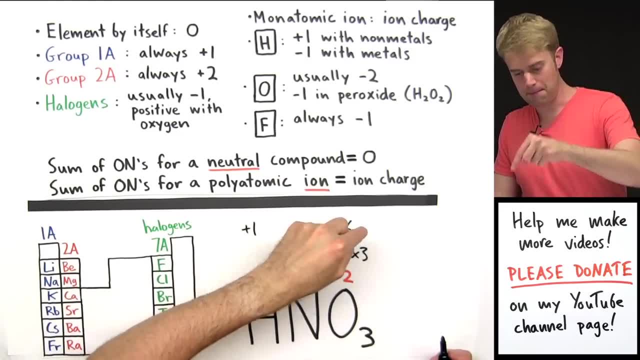 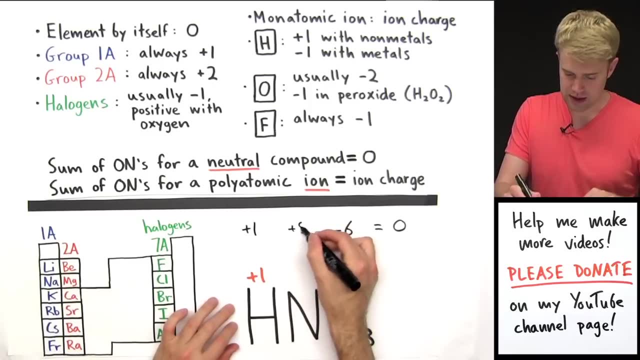 times 3 to get Minus 6.. Okay, So now we have plus 1 from the hydrogen, plus whatever nitrogen is. Minus 6 has got to give us 0 because this is a neutral compound here. So that means that in this case 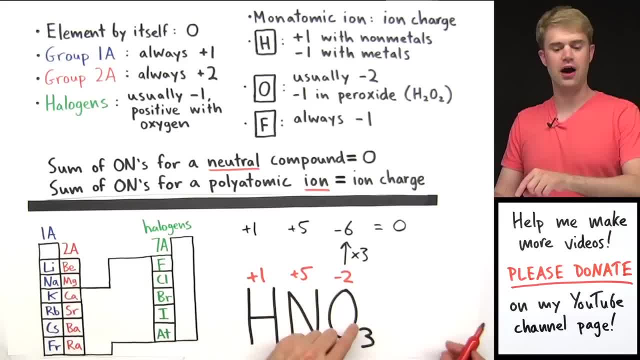 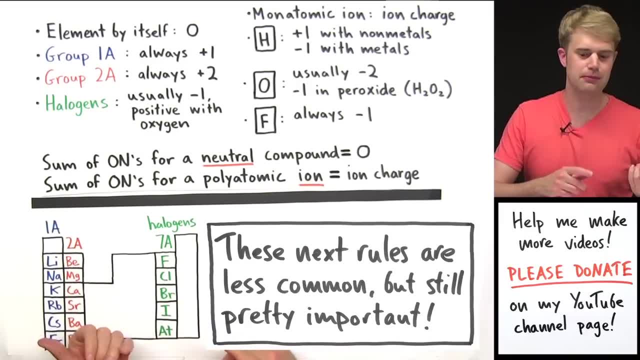 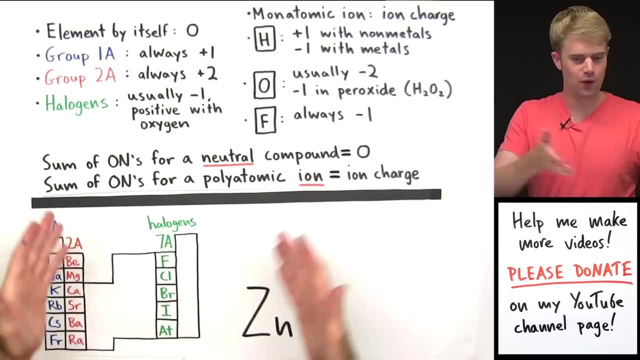 Nitrogen's oxidation number will be plus 5. 1 plus 5 minus 6 equals 0. now I'm going to start talking about some more challenging examples that use some rules here that are a little less common. ZnH2- Okay, zinc- here We don't know what its charge will be. but hydrogen- we have a rule for that now. 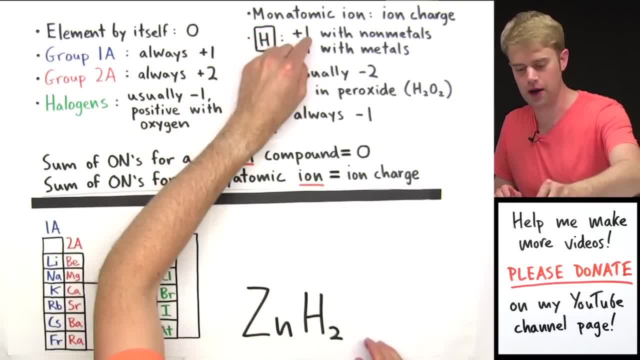 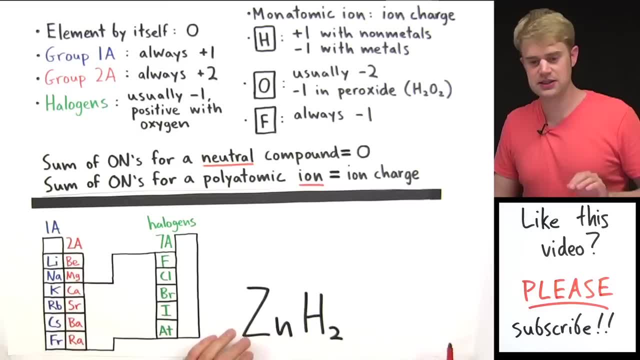 We have been used to hydrogen's number being plus 1 because it's been with nonmetals, But here it's with a metal with zinc, So that means that its oxidation number is going to be Minus 1, but we have two of these hydrogens. 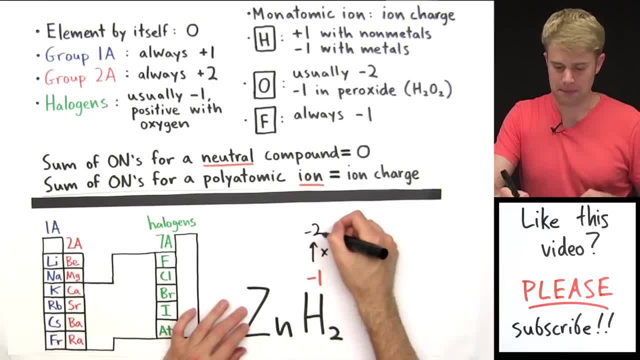 So it's going to be minus 1 times 2- give us minus 2. Since this is a neutral compound, whatever zinc is plus minus 2 has to give us 0. So that means that zinc's oxidation number must be plus 2 here. So we got plus 2 for zinc and minus 1 for hydrogen, because a hydrogen was with metal. 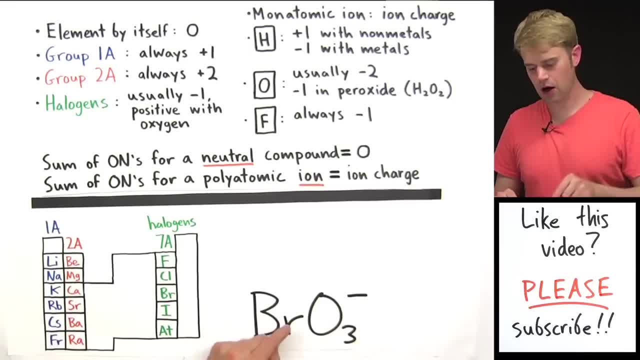 So it has a minus 1 oxidation number: BrO3- 1 minus. This is a tricky one, but it's pretty common. So Br bromine is one of the halogens. The rule for the halogens is they are usually minus 1, but they are positive with oxygen. 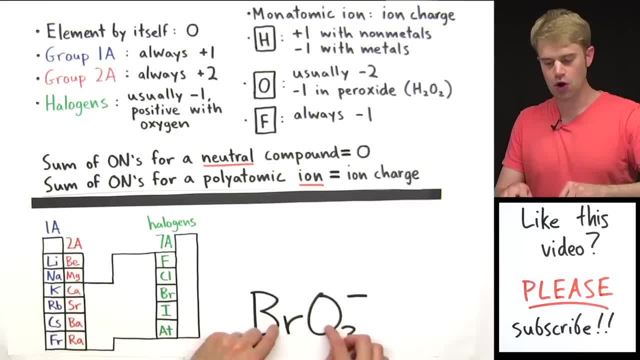 So I'm not going to put one minus in here, because it's with oxygen. So let's go to oxygen instead. Oxygen is usually minus 2, since it's not in peroxide. So let me put that here: Minus 2. now we have 3 oxygens, So that's going to be times 3 to give us. 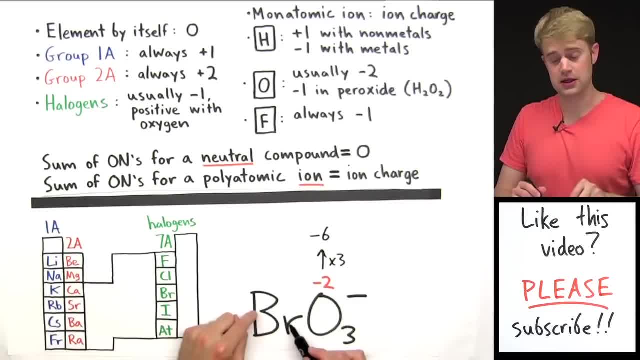 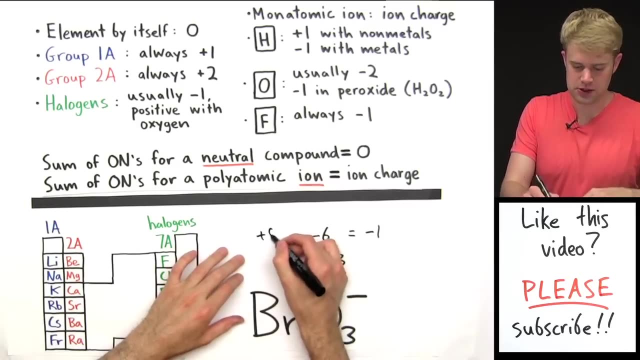 minus 6. now, whatever Bromine is Minus 6 has got to give us minus 1, because this whole thing is a polyatomic ion that has a charge of minus 1. So that means that bromine's charge must be plus 5. plus 5 minus 6 gives us. 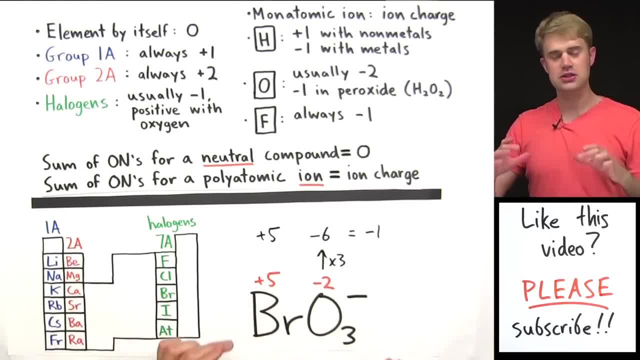 minus 1. so this is an exception where the halogens, instead of having an oxidation number of minus 1, have a positive oxidation number because they are paired up with oxygen. Keep that in mind. ClF3- Ok, so here we have 2 halogens in the same compound. 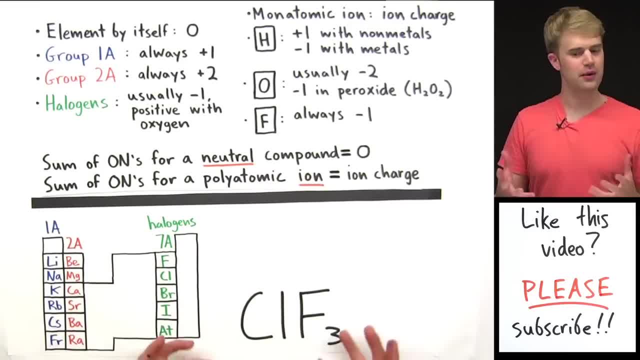 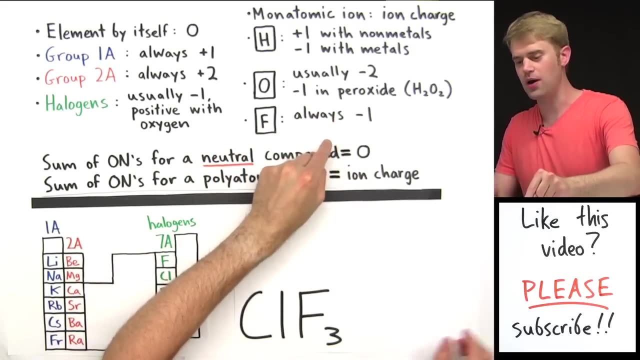 We have fluorine and chlorine. How are we going to figure this out? Well, this is one of these things that sometimes happens where fluorine combines with another one of the halogens. We're going to zero in on this rule first, that fluorine is always, always, always. 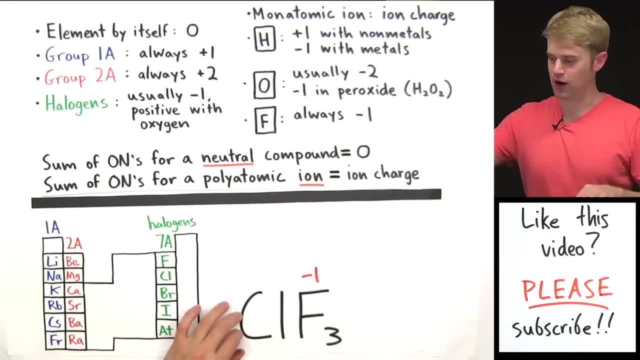 minus 1. one. so I'm gonna put a minus one right there, multiply it by three, because I have three of them, and get minus three. now chlorine, the other halogen, says that these other halogens are usually minus one, but not always they can be positive. 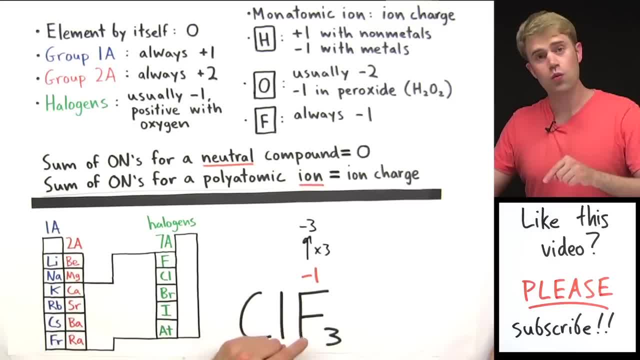 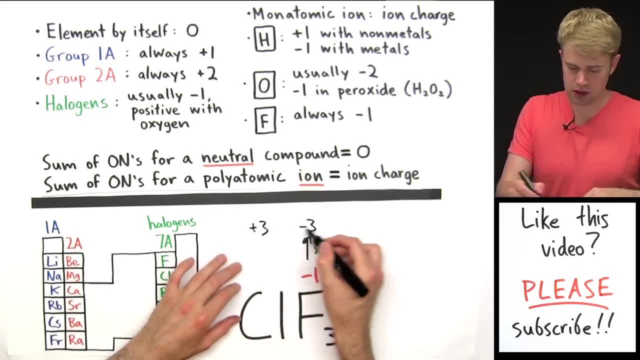 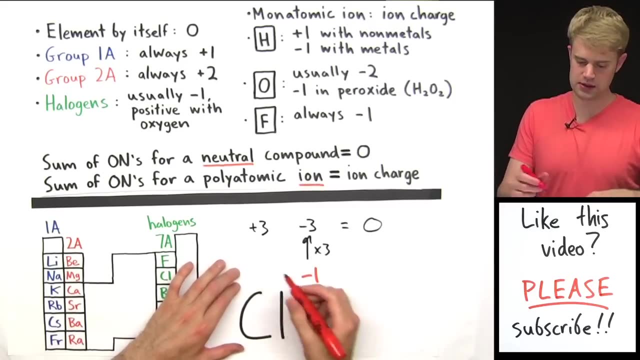 with oxygen. they can also be positive with fluorine here. so fluorine gives us minus three. chlorine must be plus three so that these can add together to give us zero, since this is a neutral compound, which means that chlorine's oxidation number must be plus three. and it's plus three instead of minus one because it's 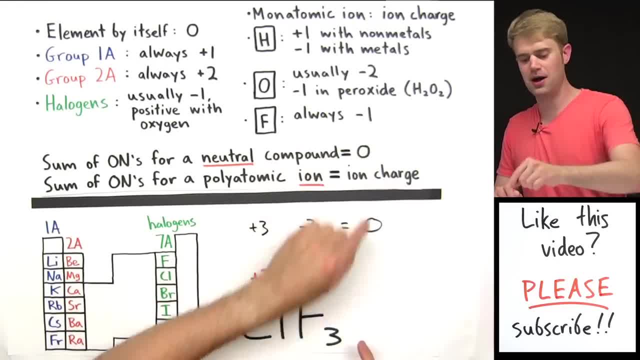 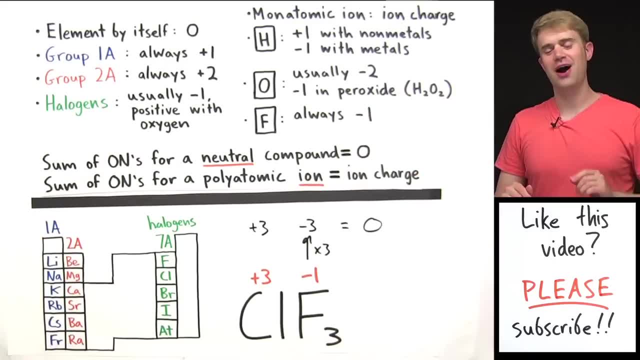 paired with fluorine, which is always, always, always minus one, no matter what. so that's how to work through these rules: to figure out what the oxidation numbers of L-chlorine and fluorine are. elements are in a compound. if you want a little bit more practice, I'm gonna have. 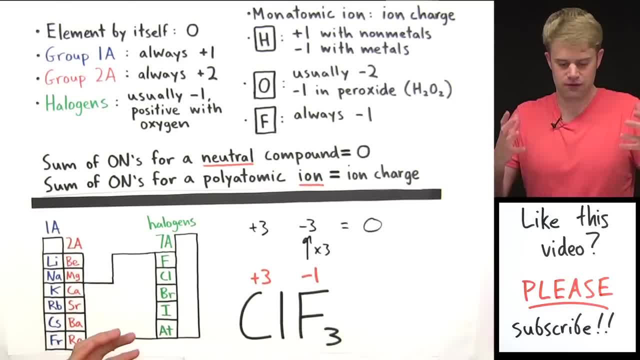 another video with more practice problems. if you just are a little bit shaky on this, doing more and more practice problems is the best way to get good really fast.